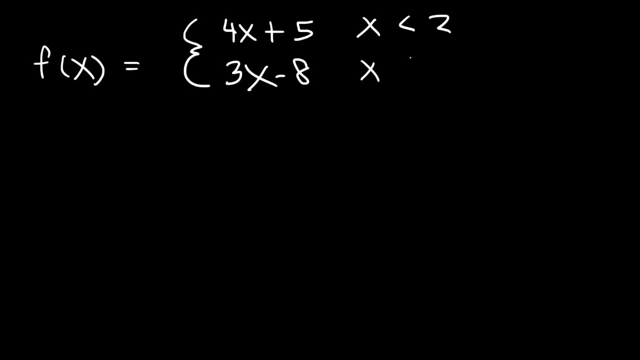 x is less than 2 and it's equal to 3x minus 8 when x is equal to or greater than 2.. So go ahead and find the value of f of negative, 2,, f of 2, and f of 5.. Feel free to pause the. 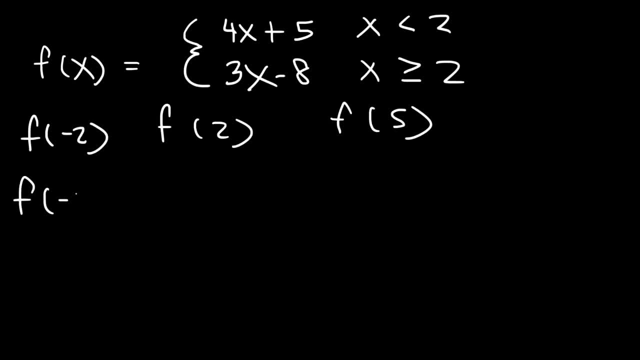 video and work on this problem. So let's evaluate the function when x is negative 2.. So should we use this portion of the piecewise function or the bottom part? Should we use 4x plus 5 or 3x minus 8? Negative 2 is less than 2.. So let's evaluate the function when x is less than 2.. 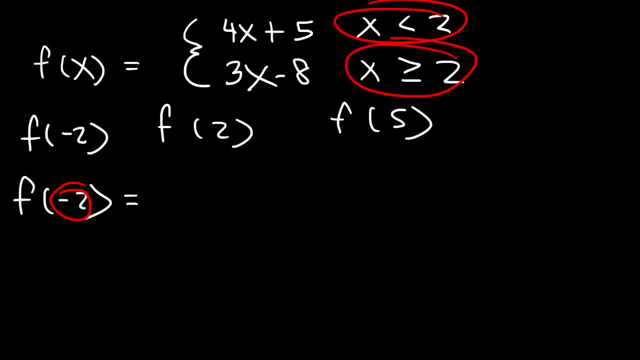 It's not equal to or greater than positive 2.. So therefore negative 2 corresponds to this range. So we need to use the first part of the piecewise function. So let's replace x with negative 2.. 4 times negative 2 is negative 8.. Negative 8 plus 5 is negative 3.. So f of 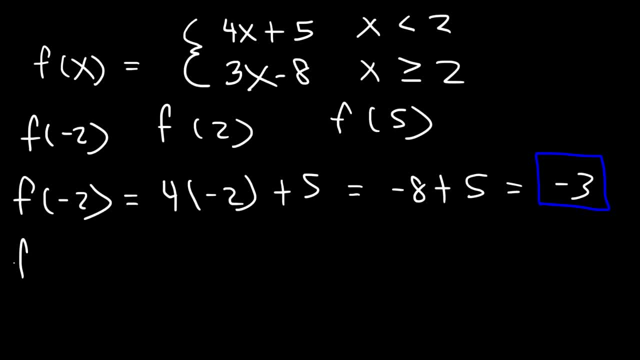 negative 2 is negative 3.. Now what about f of positive 2?? Should we use 4x plus 5 or 3x minus 8?? Now, x is equal to 2 in this equality, not in this one. So we have to use 3x minus 8.. So it's going to be 3 times 2 minus 8.. 3 times 2 is 6.. 6 minus 8 is 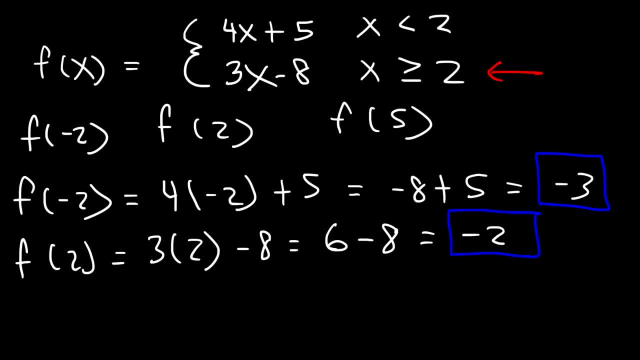 negative 2. And that's the answer. Now, what is the function value at 5?? So once again, 5 is greater than 2.. So we need to use 3x minus 8. And that's the answer. So let's evaluate the function when x is. 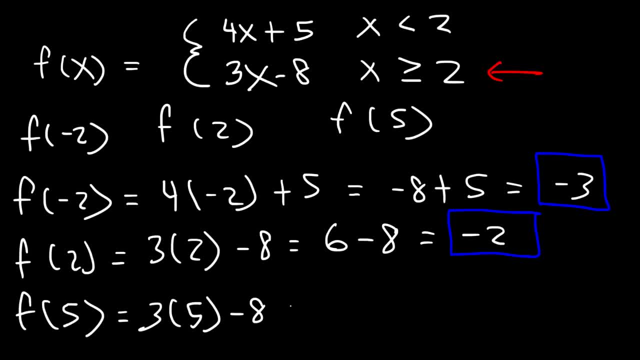 less than negative 2.. 4 times negative 2 is negative 3. So it's going to be 3x minus 8.. 🎵. 3 times 5 is 15.. 15 minus 8 is 7. And that's it. 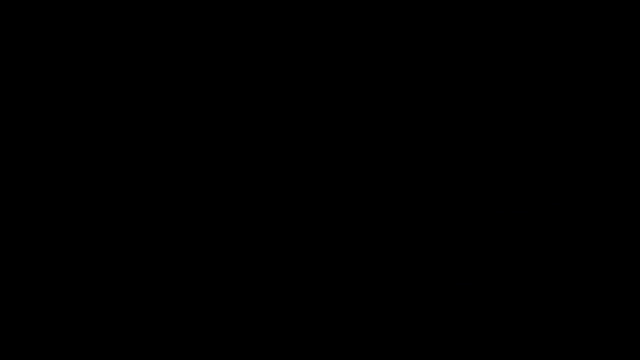 🎵. Let's work on some more examples. So let's say: if we have the function f of x and it's equal to x squared plus 3x minus 7, when x is less than negative one And it's equal to 5x plus, you can go through this and remember that you governed the second half upon after Arms 1, but you also have a function running duringỹ band 4 of sum nos 🎵, S&. All right, this is the algorithm. now that you've come to 5 and x degrees, just keep going. 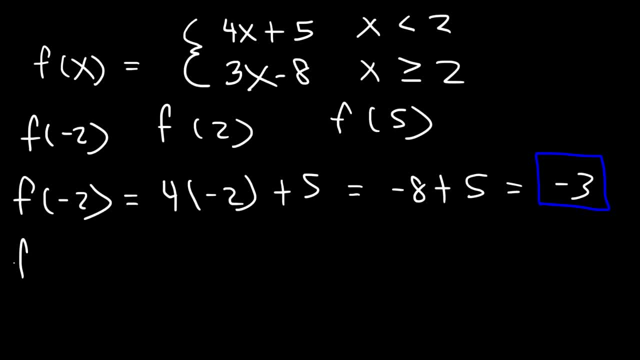 negative 2 is negative 3.. Now what about f of positive 2?? Should we use 4x plus 5 or 3x minus 8?? Now, x is equal to 2 in this equality, not in this one. So we have to use 3x minus 8.. So it's going to be 3 times 2 minus 8.. 3 times 2 is 6.. 6 minus 8 is 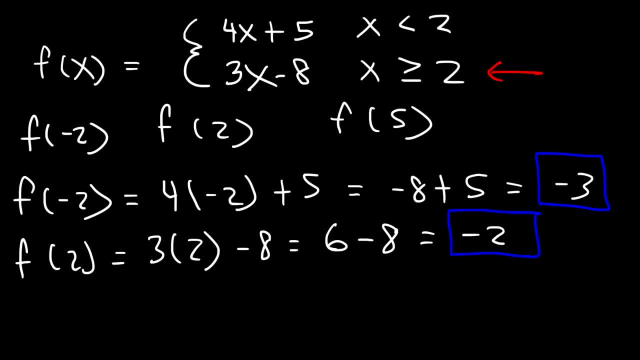 negative 2. And that's the answer. Now, what is the function value at 5?? So once again, 5 is greater than 2.. So we need to use 3x minus 8. And that's the answer. So let's evaluate the function when x is. 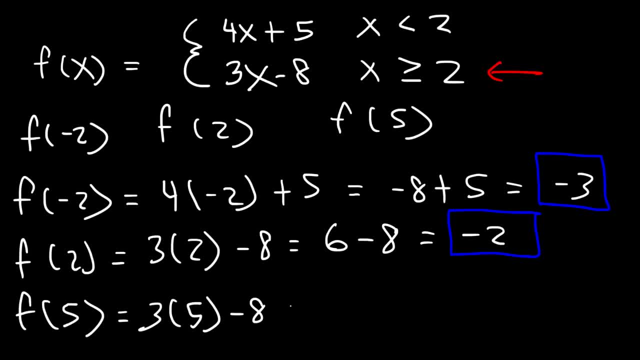 3.. So instead of 2, we have negative 3 plus 5.去 Ceatti: 5-8, 3-8.. So it's going to be 3 times 5-8.. 3 times 5: 3- 5-8.. So it's going to be 3 times 5-8.. 3 times 5-8.. 15 minus 8 is 7.. And that's it: X3, 8-8.. 15-7.. 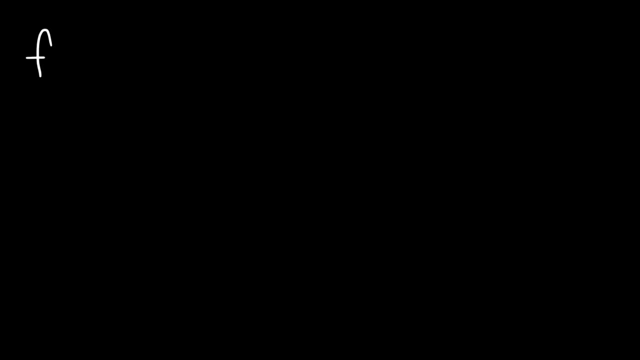 least 8.. 0-8, 17-7.. Let's work on some more examples. So let's say: if we have the function f of x, F of x and it's equal to x squared plus 3x minus 7, when x is less than negative: 1.. F of x equals: 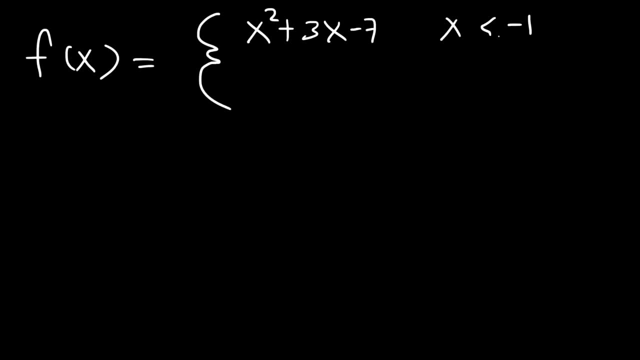 to F of x and it's equal to linear equation of the third equation. So when x is less than electric And it's equal to 5x plus 6 when x is greater than or equal to negative 1.. Actually, let me change that. 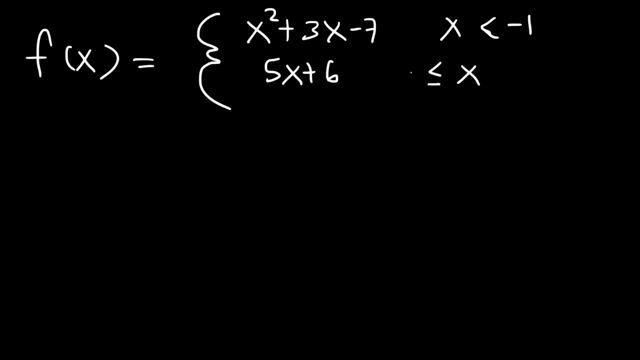 Let's say when x is greater than or equal to negative 1, but less than 2.. And let's say it's equal to x cubed plus 4 when x is greater than 2.. And it's equal to 12 when x equals 2.. 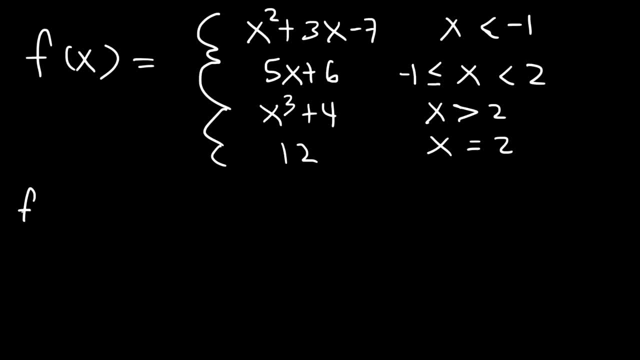 So, with this information, I want you to evaluate f of negative 4, f of, let's say, 0, f of 2, and f of 3.. So feel free to pause the video and try that. So let's evaluate. 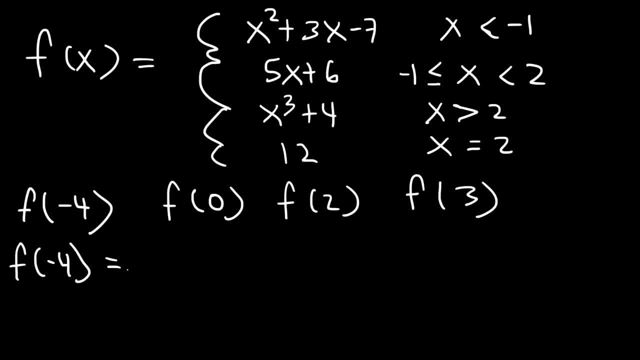 Let's evaluate the function at: x equals negative 4.. So negative 4 is less than negative 1. Therefore, we need to use x squared plus 3x minus 7.. So this is going to be negative 4 squared plus 3 times negative 4 minus 7.. 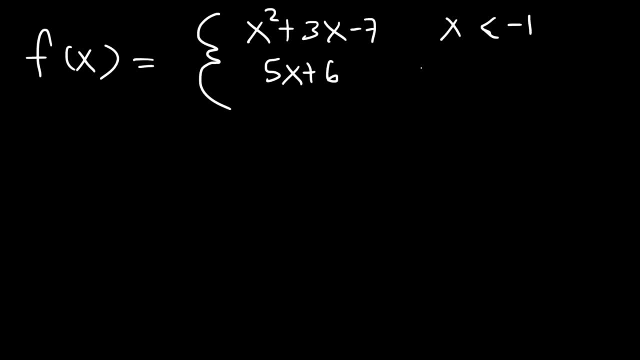 And then you could model it later if you were limited by anything else. okay, And let's do some equal to 5x plus 6 when x is greater than or equal to negative 1. actually, let me change that. let's say when x is greater than or equal to negative 1, but 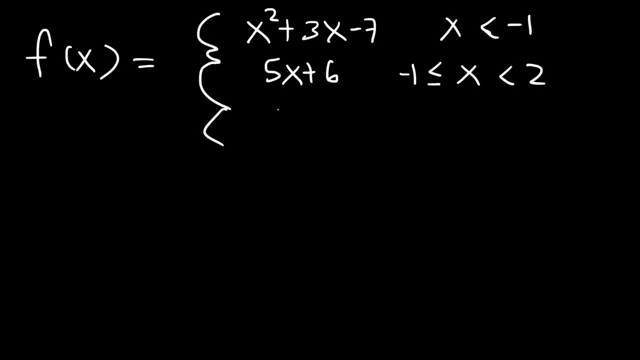 less than 2 and let's say, it's equal to x cubed plus 4 when x is greater than 2, and it's equal to 12 when x equals 2. so with this information, I want you to evaluate f of negative 4, f of, let's say, 0, f of 2 and f of 3. so feel free to pause. 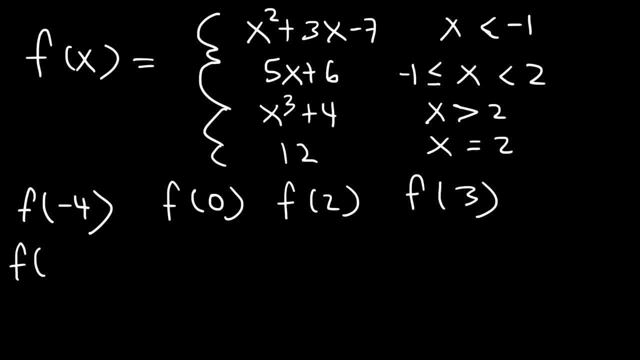 the video and try that. so let's evaluate the function at. x equals negative 4, so negative 4 is less than negative 1. therefore, we need to use x squared plus 3x minus 7, so this is going to be negative 4 squared plus 3 times negative 4 minus 7, negative 4 squared, or. 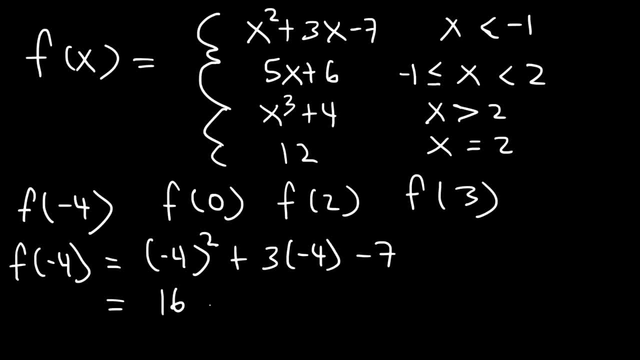 negative 4 times negative 4, that's 16, 3 times negative. 4 is negative 12, and 6 minus 12 is 4. 4 minus 7 is negative 3. so f of negative 4 is equal to negative 3. so 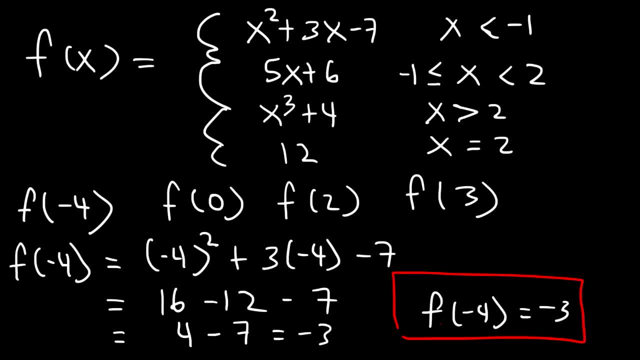 that's the first answer. I believe my math is correct. I don't think I made any mistakes on that. now let's evaluate f of 0. 0 is between negative 1 and 2, so we need to use 5x plus 6. so this is going to be 5 times 0 plus 6. 5 times 0 is. 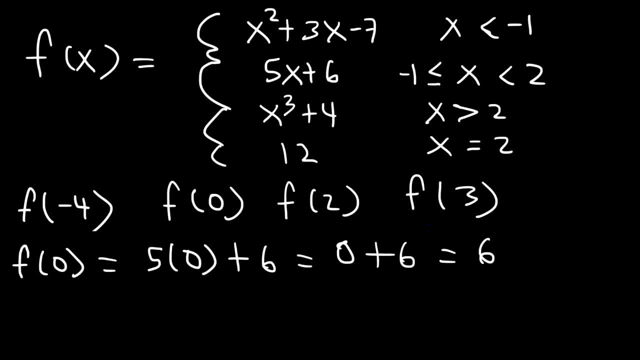 0, 0 plus 6 is 6. now what about the next one, f of 2? now, when x is exactly 2, the function is equal to 12, so f of 2 is 12. there is no math involved in that step. now what? 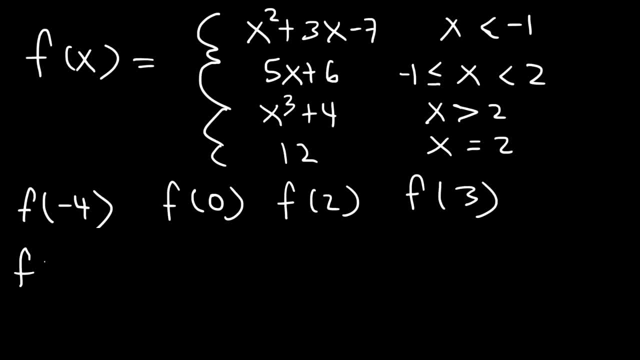 out the last one, f, of 3. when x is 3, we need to use x cubed plus 4, because that's when x is greater than 2, when x is 3. so therefore this is going to be 3 raised to the third power plus 4, so 3 to the. 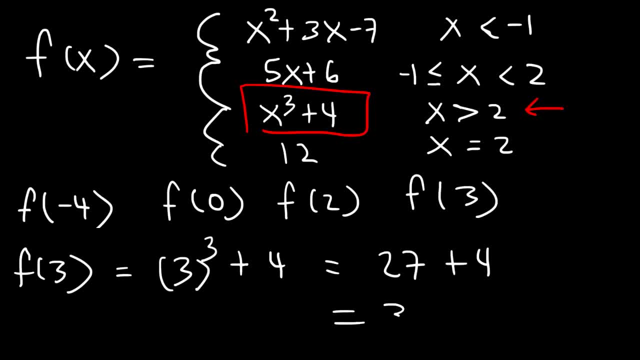 third power is 27. 27 plus 4 is equal to 31, and that covers that problem. 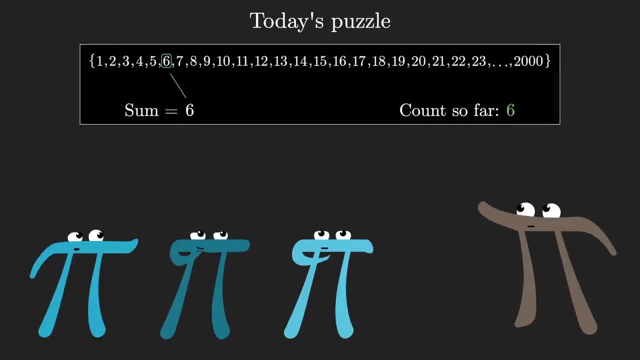 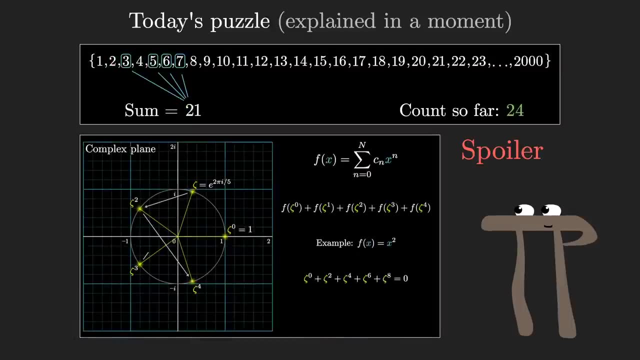 In a moment, I will ask you a puzzle, and it's a pretty hard puzzle actually. But before I do, I want to lead with a spoiler, which is the fact that the way we're going to solve this involves the use of complex numbers, And once you hear it, you will agree that that seems absurd. 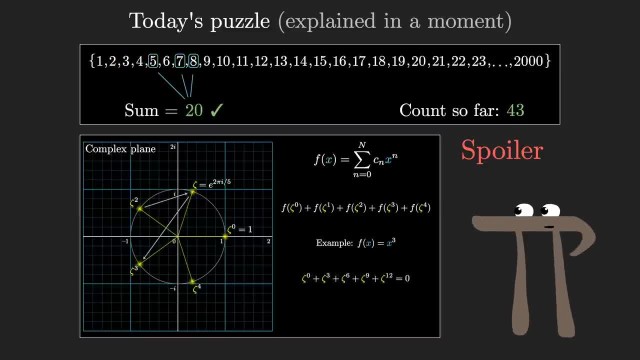 given that the puzzle is going to be purely a discrete question, It only asks about whole numbers and their sums. There's not a whiff of the imaginary, or even continuity, anywhere on the horizon. It's certainly not the only time that complex numbers are unreasonably useful for 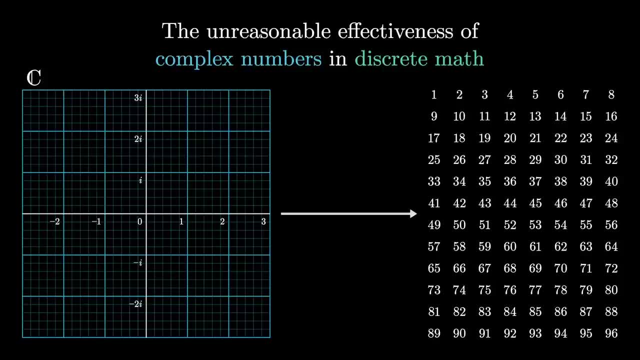 discrete math, to borrow a phrase. The more famous example that I could bring up would be how, the modern way that mathematicians understand prime numbers. you know questions about how they're distributed, their density at certain regions, things like that. well, it involves studying. 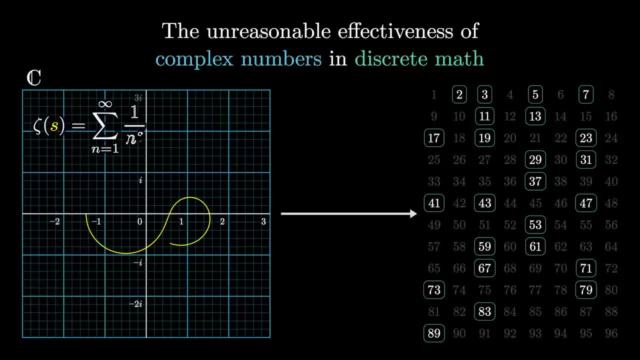 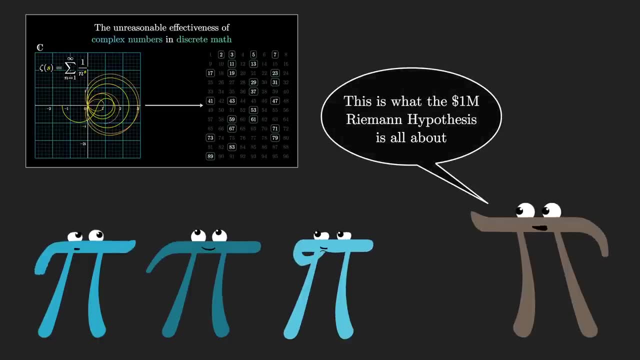 specially designed functions whose inputs and outputs are complex numbers. Some of you may know that this is what the famous Riemann hypothesis is all about. Basically, there's a specially designed function and on the face of it it looks unrelated to the discrete world.